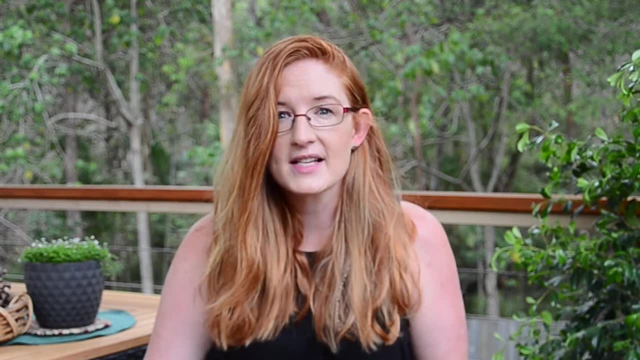 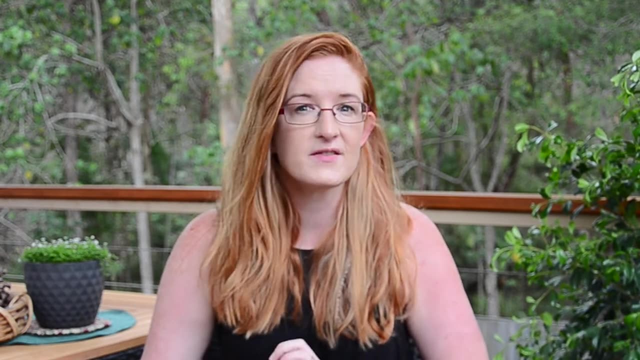 more important than ever. The most convincing reason to get your kids outside more is that it significantly improves all aspects of child development: physical, cognitive, social and emotional. If you want to learn more about outdoor play, please visit our website at wwwoutdoorplaycom. 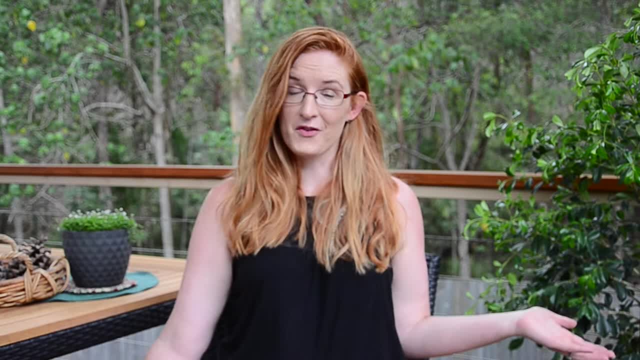 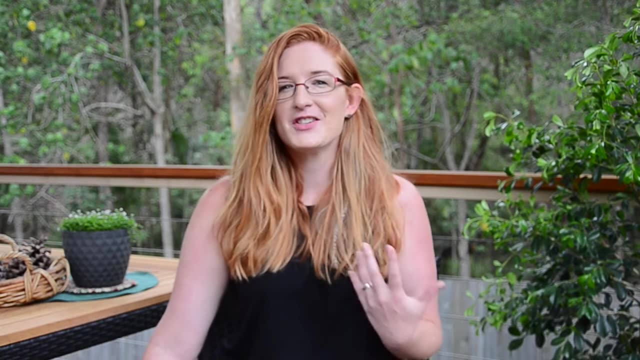 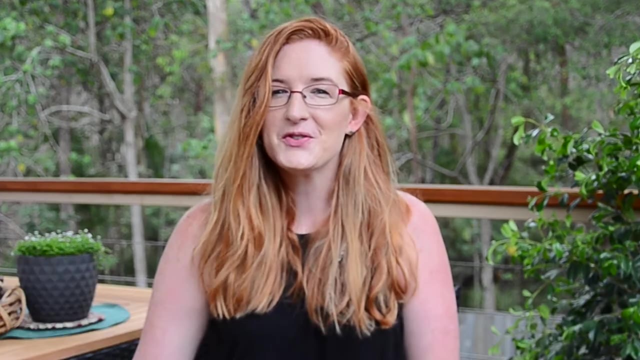 Playing outdoors grows your child's resilience, self-confidence, initiative, creativity and more. It encourages the joy of movement. it nurtures friendships, social connections and stimulates their imagination and promotes experimentation. Children feel better when they spend time in nature. Don't just take my word from it. A growing number of studies and recommendations. 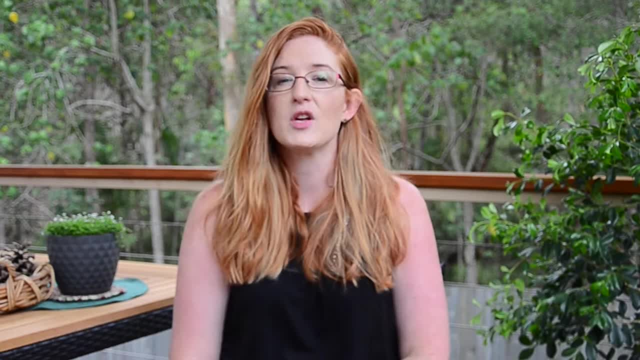 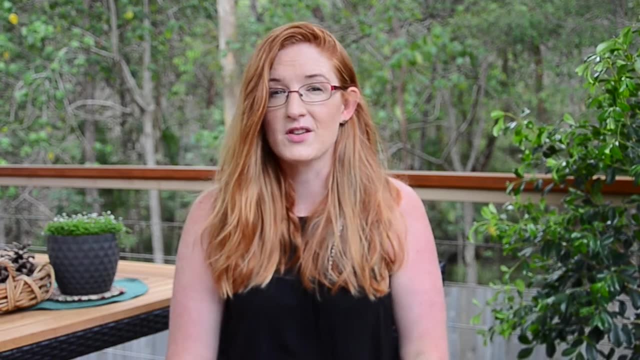 from doctors, mental health experts, educational experts and occupational therapists agree that outdoor play is important. I've linked to the Children and Nature Network below if you'd like to do your own research. There's heaps of studies there that tell you the benefits of outdoor play. 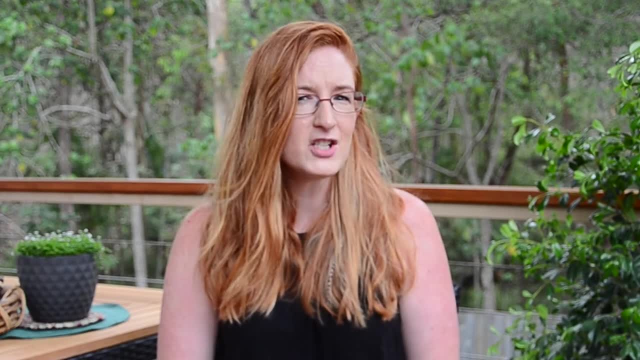 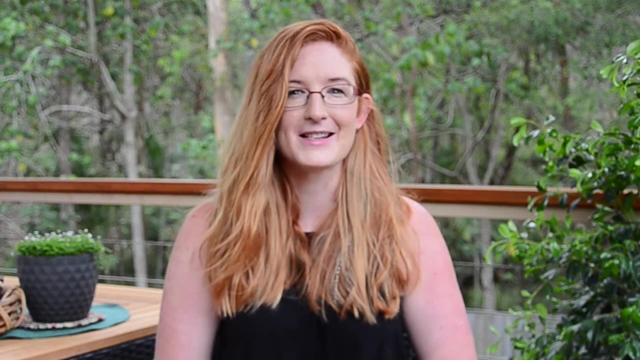 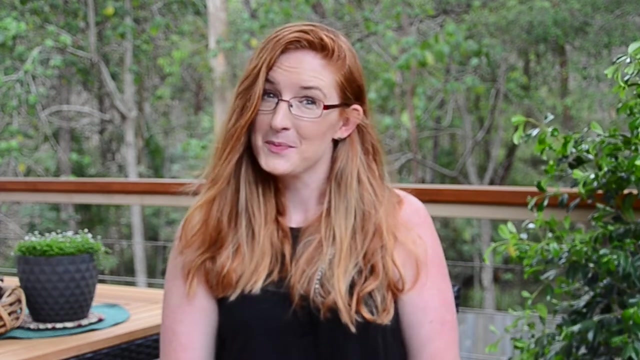 and playtime in nature. Now you might be asking: is nature play only for children? Well, in my opinion, nature play, or outdoor play, is available to everyone and benefits everyone. I certainly play differently outside to that of my children, but I do play, I weave, using natural. 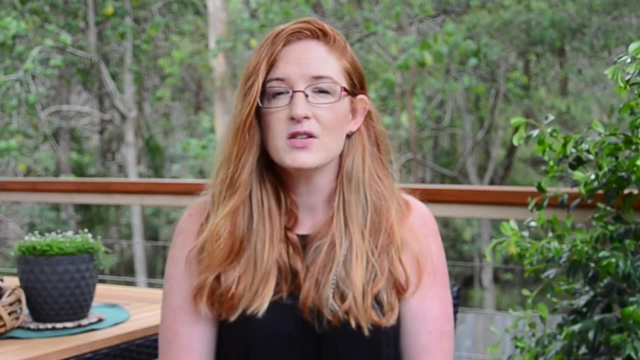 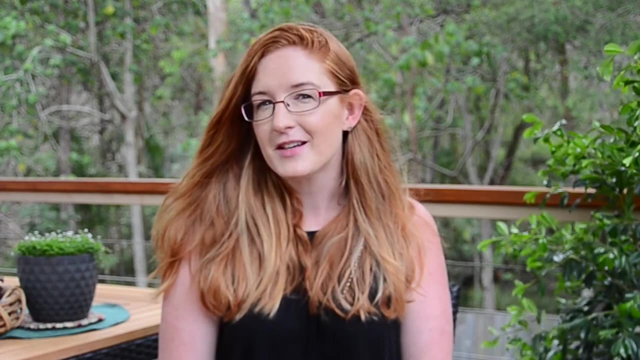 materials. I stroll around my garden and look at the plants, and I get into a peaceful contemplative zone when I'm watching a spider craft its web. My children, on the other hand, are a little bit different. They make forts and play in their mud kitchen and roll down grassy. 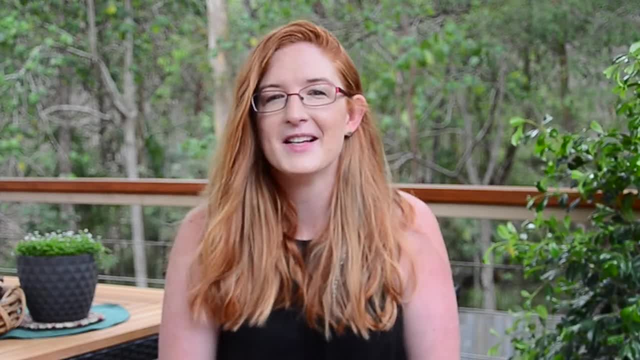 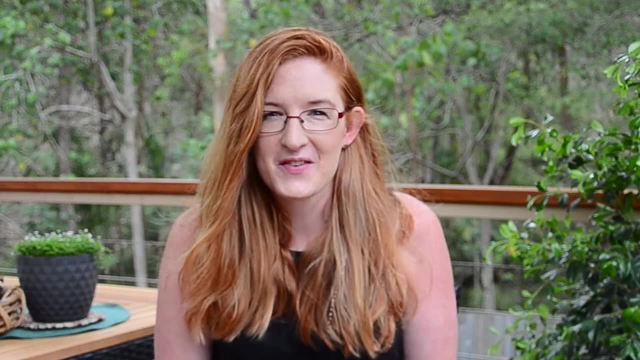 hills when they find one. They're a little bit more active than I am. Together, though, we enjoy crafting with nature, walking in the nature reserve behind our home and inviting friends over to enjoy our backyard with us. If I've convinced you, how do you get? started. How do you get your children outside more often? This one's pretty obvious, but number one is: go outside with your child. Don't force your child out if they don't want to go though. Instead, just encourage them out with a simple task to perform together. They love being with. 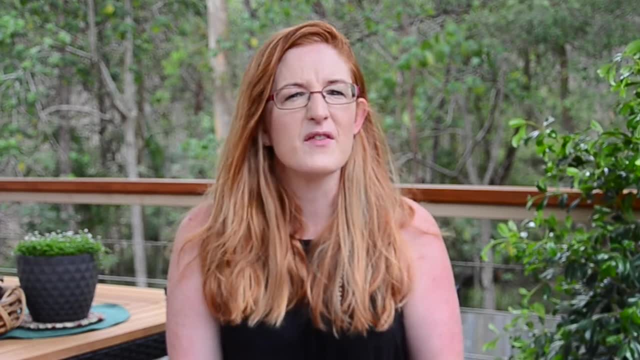 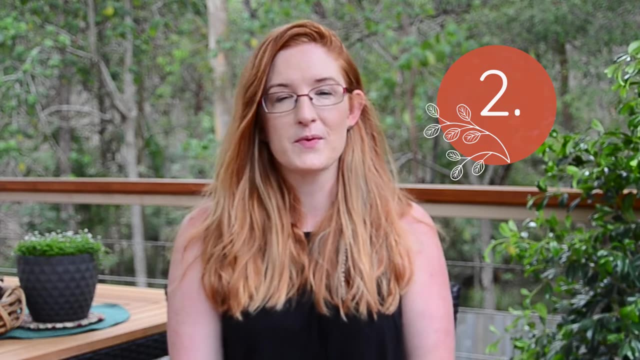 you, and it's a really easy way to convince them to come out And be sure to let them finish what they're already doing as well. The second tip is to go anywhere as long as it's outside, So nature is all around us. Even in the city, you can find little green spaces. 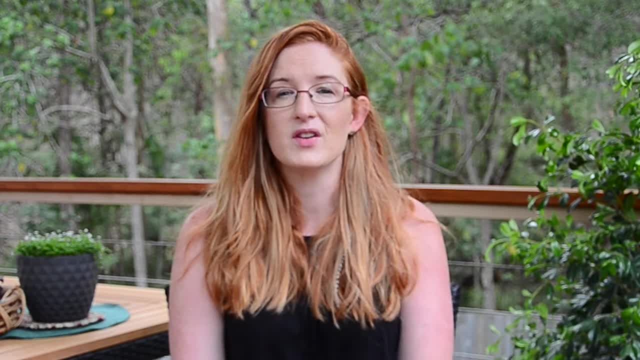 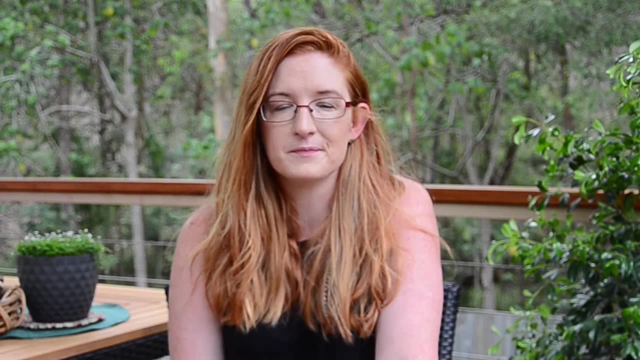 and sometimes you only have to look up at the clouds or feel the breeze on your skin to find it, Although I would recommend a natural setting, as this is where the benefits are provided in full. The third tip is to keep it simple. If you're only starting out, don't make it complicated.